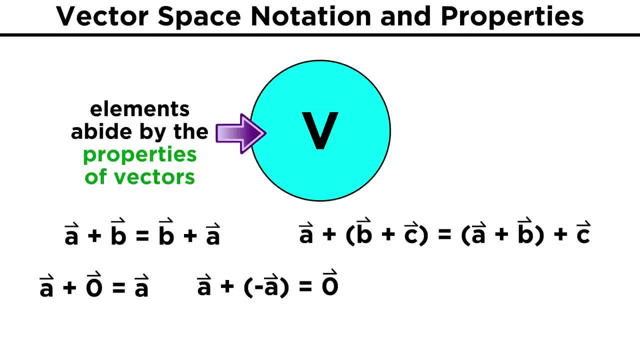 vector will just give back the element. For each element A, there exists another element, negative A, within V, such that the addition of the two gives the zero vector. Scalars can be distributed across the addition of two members of V. The product of two scalars multiplied by an element is the same as one of the scalars. 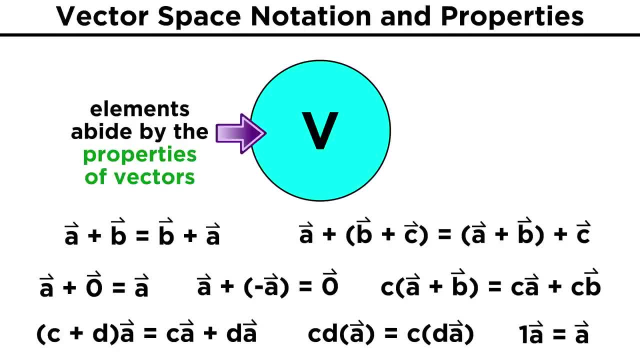 times the product of the other scalar and the element And finally, multiplying by the scalar, one just gives back that element. So these are simply properties that elements of the vector space must possess, and in this way we can regard a vector space as a vector space. 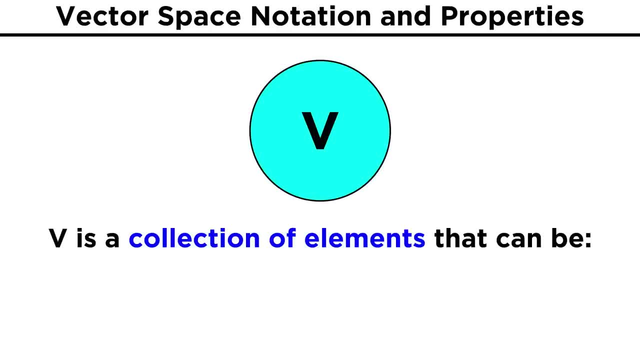 We can regard a vector space as a collection of elements that can be added together in any combination and multiplied by scalars in any combination. Now, an important property of a vector space is something called closure. Closure requires two properties. First, for an element A of V, multiplying A by any scalar will give a result that is: 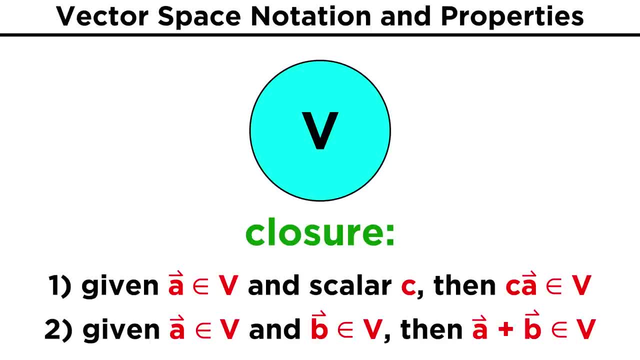 also within V. Second, for any two elements- A and B- within V, adding the two elements will also give a result that is contained within V. These closure properties are what determine if V is a vector space. Let's take some time to examine these properties. 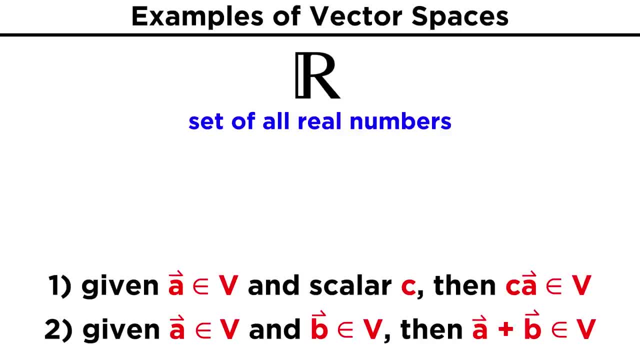 At this point, it will be useful to introduce this R symbol, which represents the set of all real numbers, meaning positive, negative, rational, irrational and non-negative, For example, all the real numbers we talked about when we discussed the types of numbers. 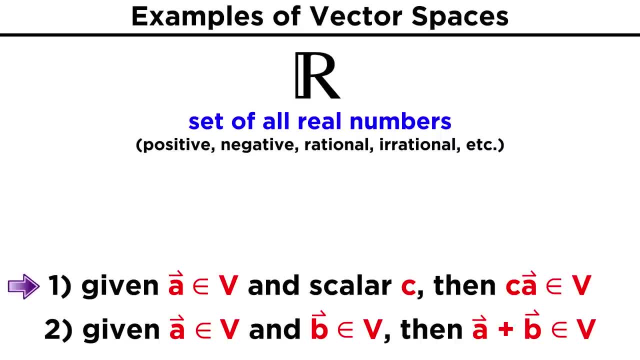 in a previous tutorial. We can pick any element of this, set a real number and multiply it by any scalar we want. Let's take the number five as our element and multiply it by a few scalars. Two times five is ten. 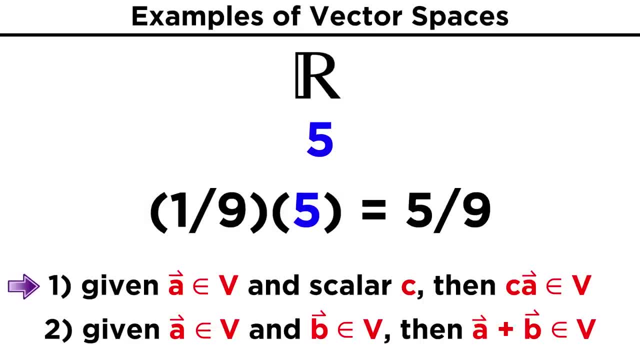 Eight thirds times five is forty thirds. One ninth times five is five ninths Pi times five is five pi and so on. Notice that all of our results are still real numbers. This is because, no matter what we choose, a real number times a real number is still. 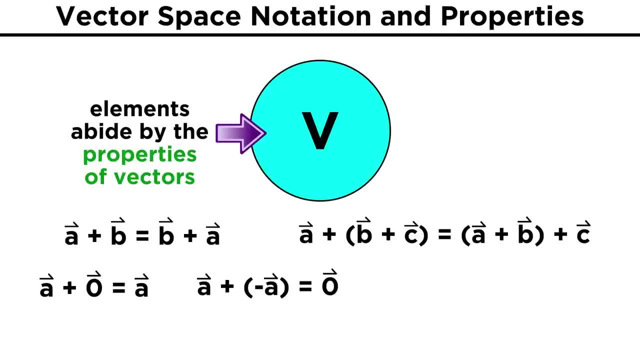 For each element A, there exists another element, negative A, within V, such that the addition of the two gives the zero vector. 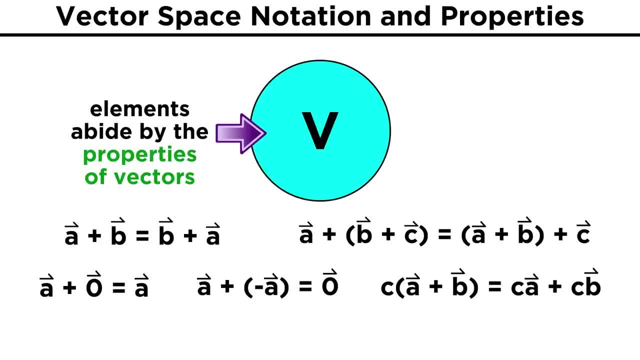 Scalars can be distributed across the addition of two members of V. Just as an element can be distributed across the addition of two scalars. The product of two scalars multiplied by an element is the same as one of the scalars 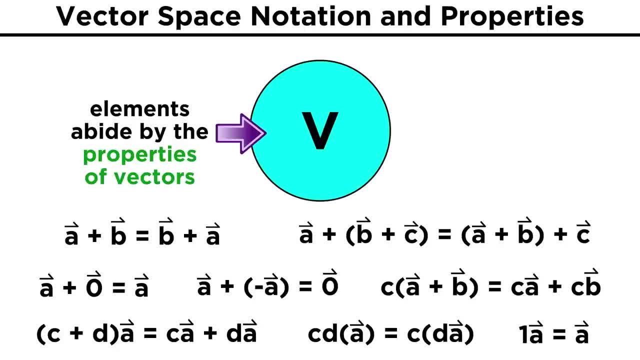 times the product of the other scalar and the element. 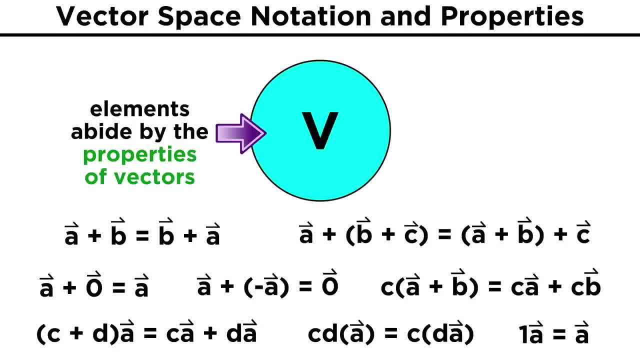 And finally, multiplying by the scalar one just gives back that element. 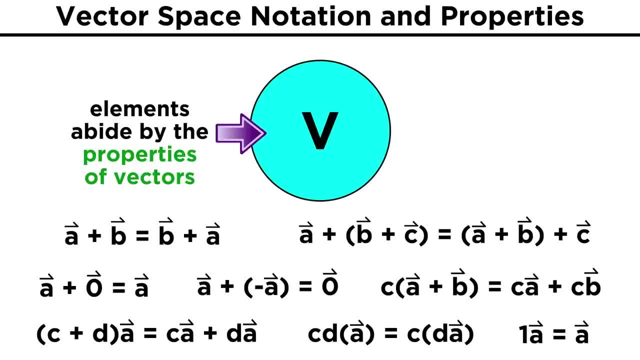 So these are simply properties that elements of the vector space must possess, and in this way, we can regard a vector space as an element. 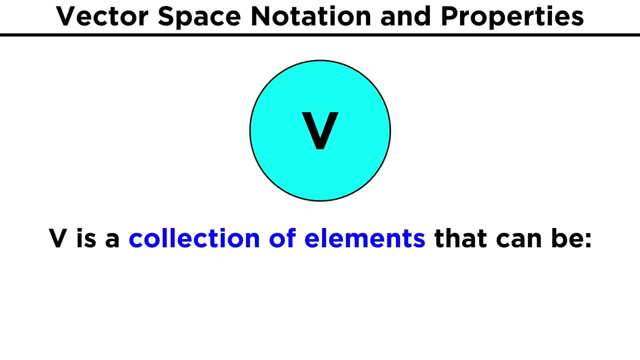 We can regard a vector space as a collection of elements that can be added together in any combination and multiplied by scalars in any combination. Now an important property of a vector space is something called closure. Closure requires two properties. First, for an element A of V, multiplying A by any scalar will give a result that is also within V. 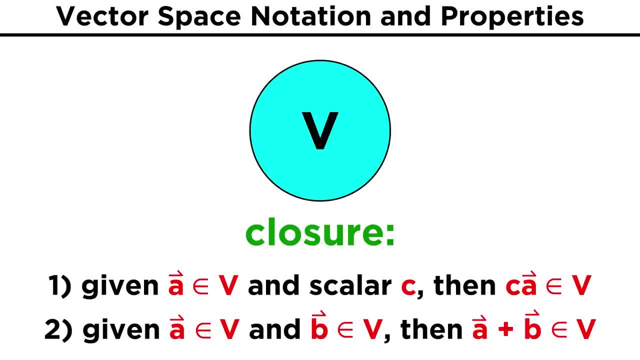 Second, for any two elements A and B within V, adding the two elements will also give a result that is contained within V. These closure properties are what determine if V is a vector space. 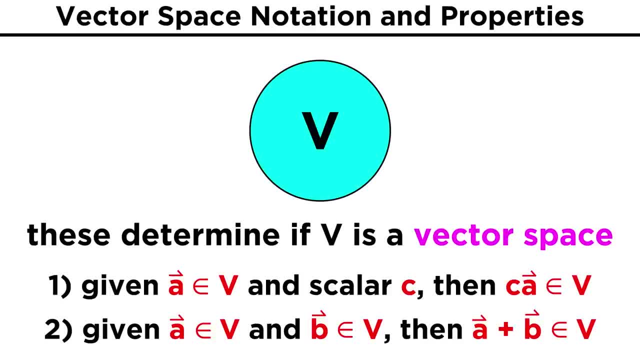 Let's take some time to examine these properties. At this point it will be useful to introduce this R symbol, which represents the set of all real numbers, meaning positive, negative, rational, irrational, and non-negative. 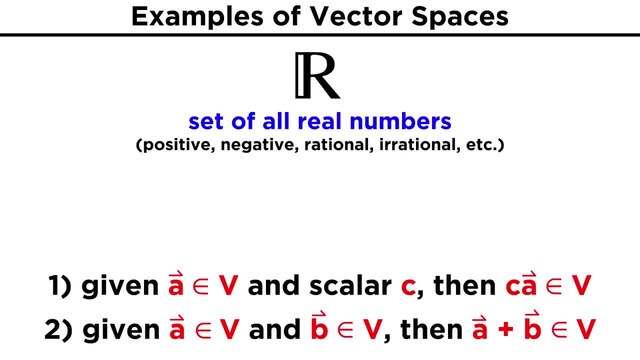 Now, all the real numbers we talked about when we discussed the types of numbers in a previous tutorial. 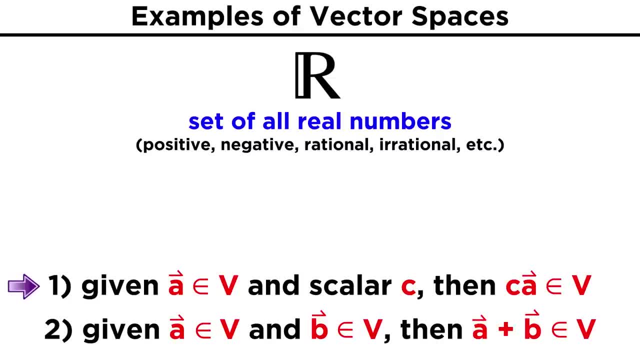 We can pick any element of this set, a real number, and multiply it by any scalar we want. 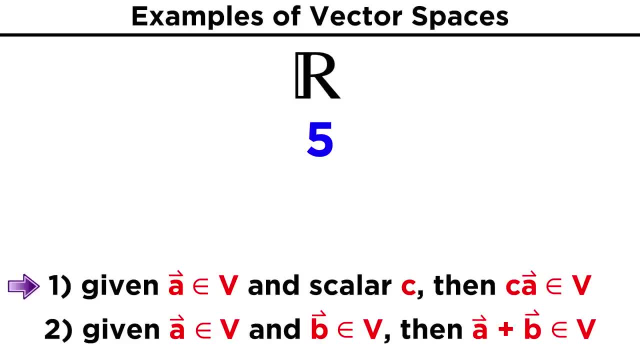 Let's take the number five as our element, and multiply it by a few scalars. Two times five is ten. Eight thirds times five is forty thirds. One ninth times five is five ninths. Pi times five is five pi, and so on. Notice that all of our results are still real numbers. This is because no matter what we choose, a real number times a real number is still real. So the set of real numbers satisfies the first closure property. 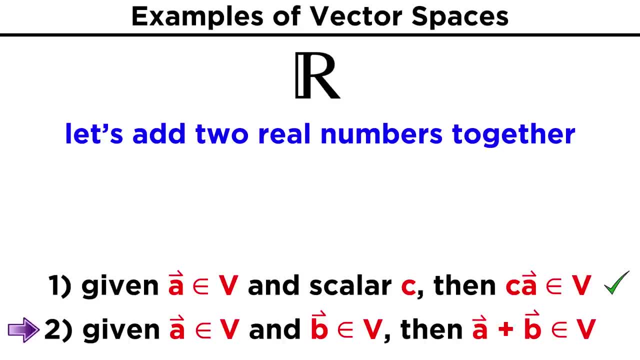 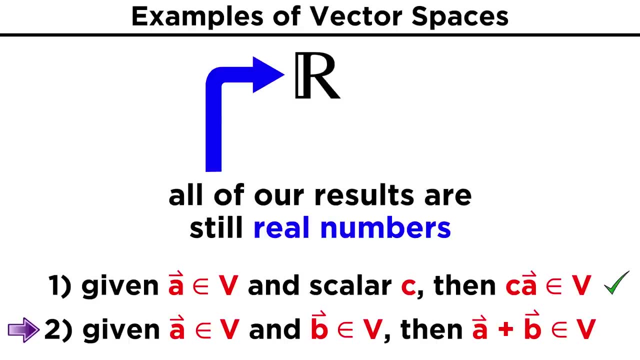 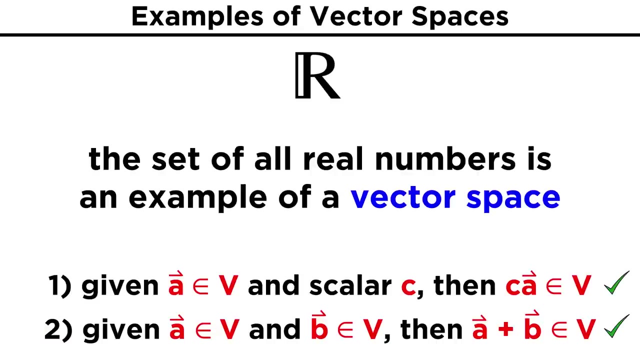 Now for the second property, we will need to choose two elements to add together. We could choose seventy-four and negative ten, adding them together to get sixty-four. Adding two and four fifths. Gives us fourteen fifths. No matter what two real numbers we choose, the sum of two real numbers is still real, so because the two criteria have been met, the set of real numbers is closed and can be considered a vector space. 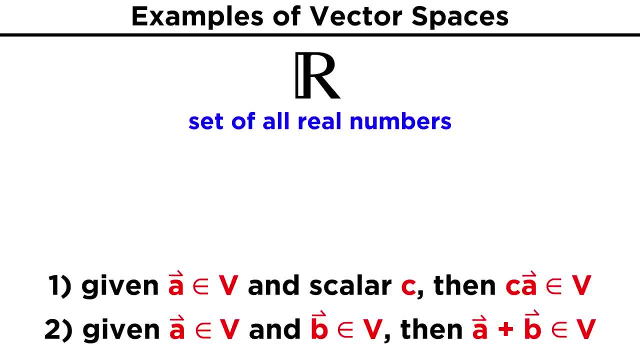 Moving to another example, let's expand on our notation. If R is the set of real numbers, Rn is the set of real vectors with a length of some integer n. 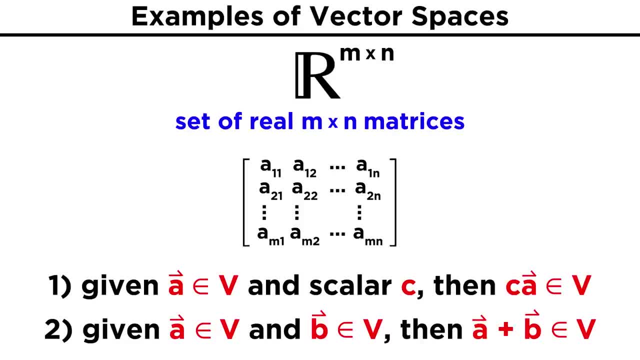 Similarly, RM by n is the set of real m by n matrices. 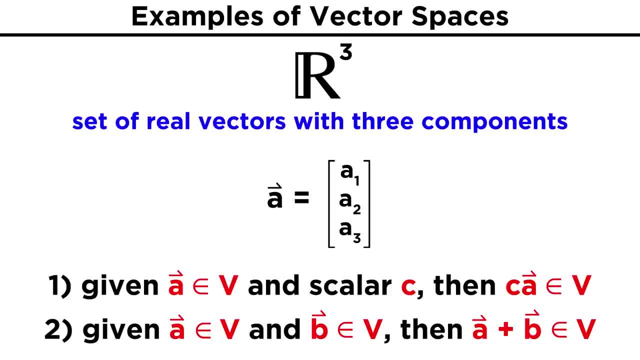 First, let's just look at R3 vectors. We can multiply any such vector by any scalar, and find that our result is a vector of length three, made of real numbers. 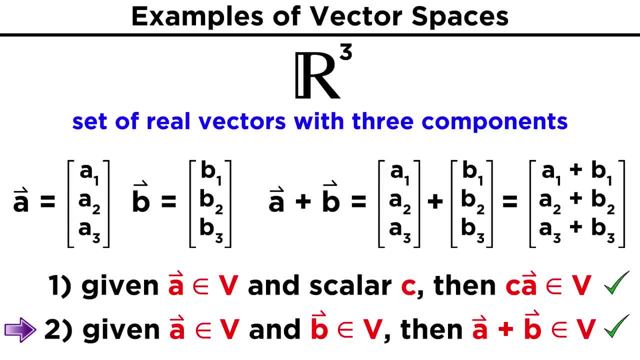 Similarly, we can add any two elements and find the same to be true, given that each component is simply now a sum that will result in a vector of length three. Similarly, we can add any two elements and find the same to be true, given that each component is simply now a sum that will result in a vector of length three. result in another real number. 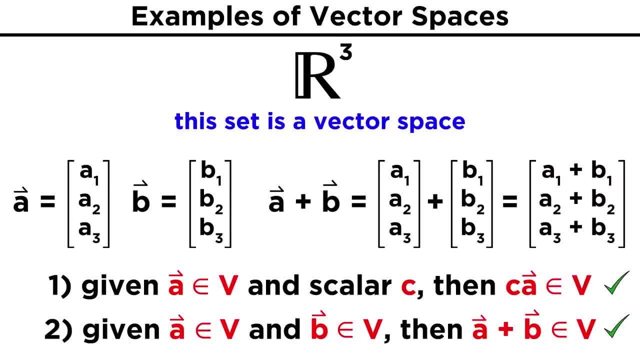 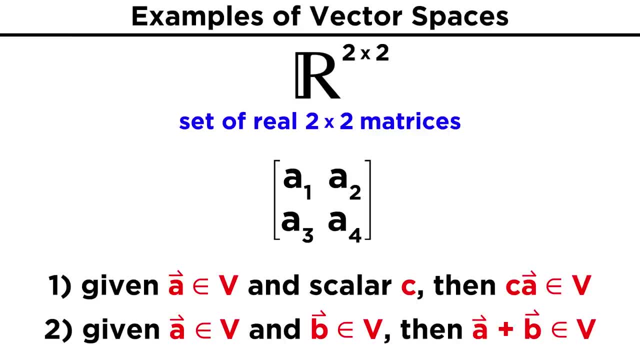 This set is closed, and is thus also a vector space. Given what we know about matrix addition, if some set is comprised of matrices with the same dimensions, multiplying by some scalar, or adding any two matrices together will not change their dimensions, which makes this two a vector space. 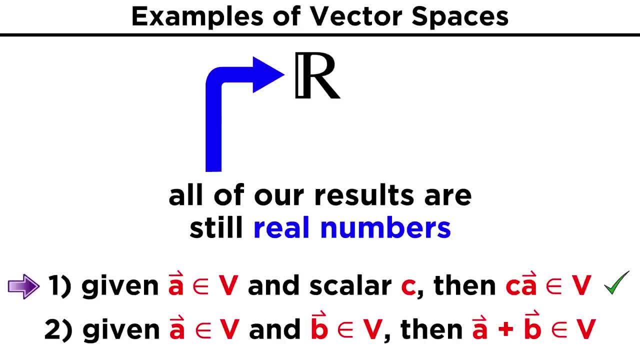 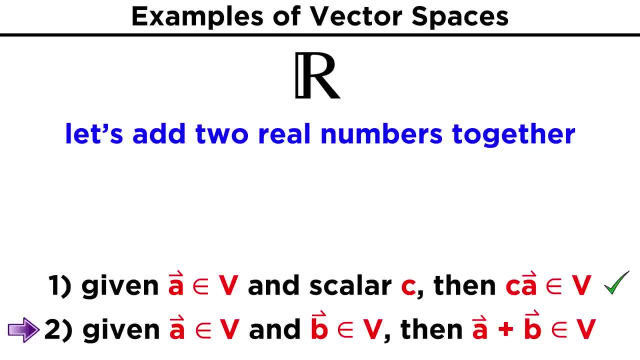 real. So the set of real numbers satisfies the first closure property. Now for the second property. we will need to choose two elements to add together. We could choose seventy-four and negative ten. adding them together to get sixty-four. Adding two and four-fifths: adding them together to get sixty-four. 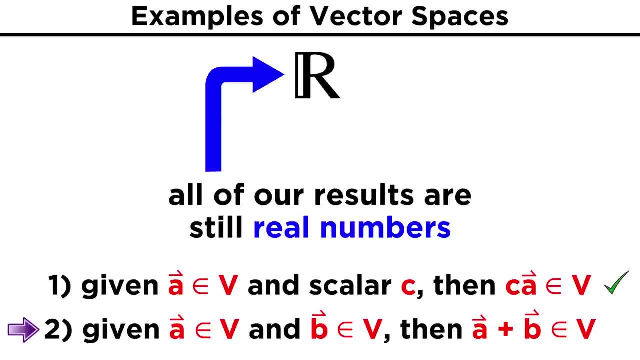 Adding two and four-fifths, adding them together to get sixty-four. Adding two and four-fifths gives us fourteen-fifths. No matter what two real numbers we choose, the sum of two real numbers is still real. so because the two criteria have been met, the set of real numbers is closed and can. 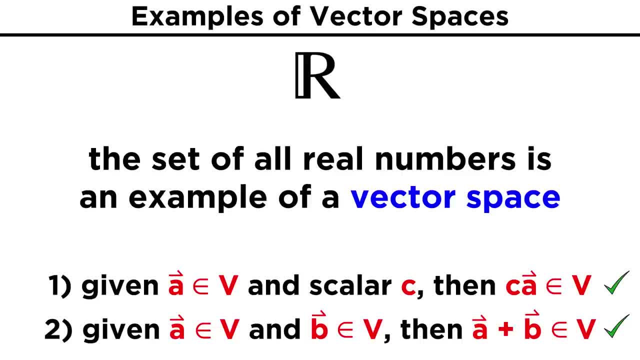 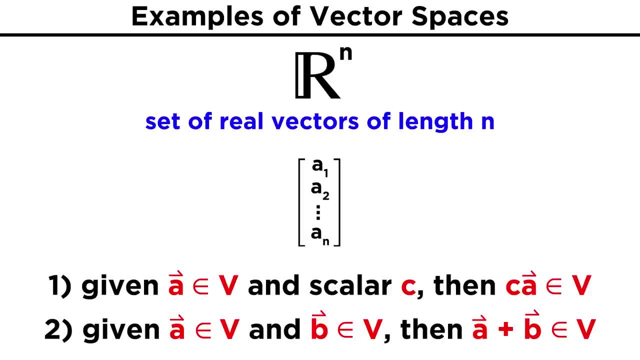 be considered a vector space. Moving to another example, let's expand on our notation. If R is the set of real numbers, Rn is the set of real vectors with a length of some integer n. Similarly, Rm by n is the set of real m by n matrices. 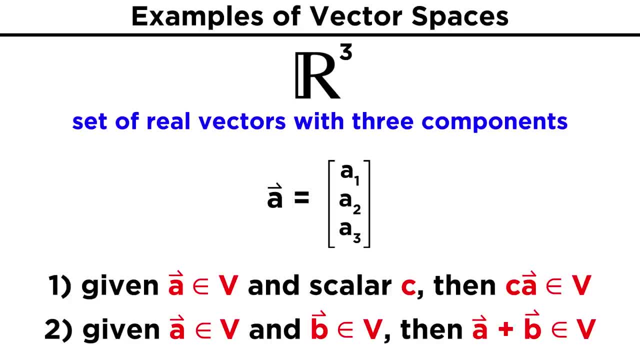 First, let's just look at our three vectors. We can multiply any such vector by any scalar and find that our result is a vector of length three, made of real numbers. Similarly, we can add any two elements and find the same to be true, given that each. 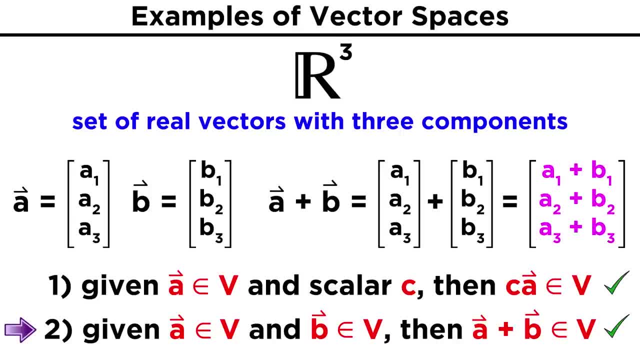 component is simply now a sum that will require a sum. What does that mean? result in another real number. This set is closed and is thus also a vector space, Given what we know about matrix addition, if some set is comprised of matrices with 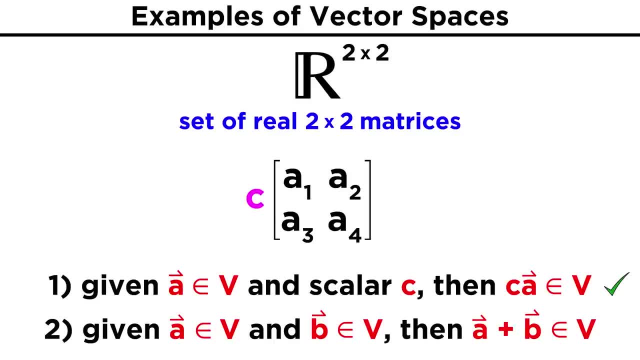 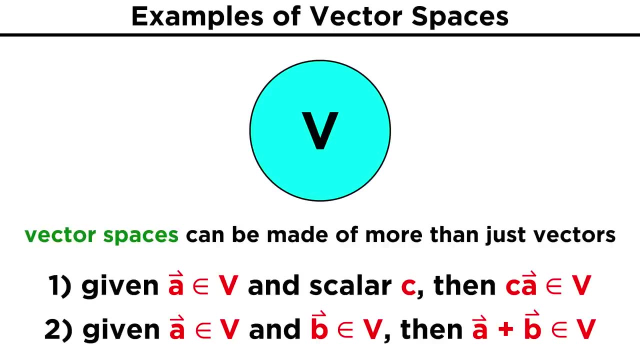 the same dimensions. multiplying by some scalar or adding any two matrices together will not change their dimensions, which makes this two a vector space. So it would seem that vector spaces can actually be made of more than just vectors. In fact, we could define a vector space that was made up of functions if we wanted to. 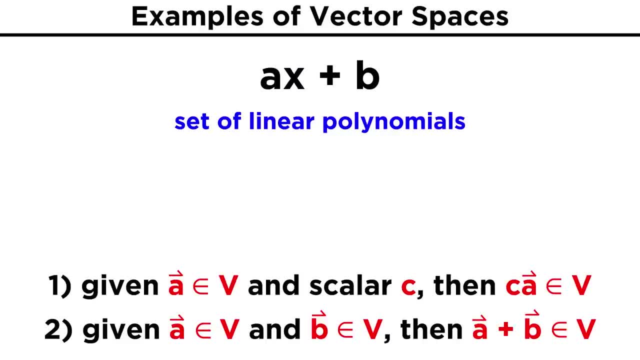 For example, let's take the set of linear polynomials in the form of AX plus B. If we multiply by a scalar C, we can distribute to get CA times X plus BC. Since we are dealing with real numbers, CA and BC will also be real numbers. 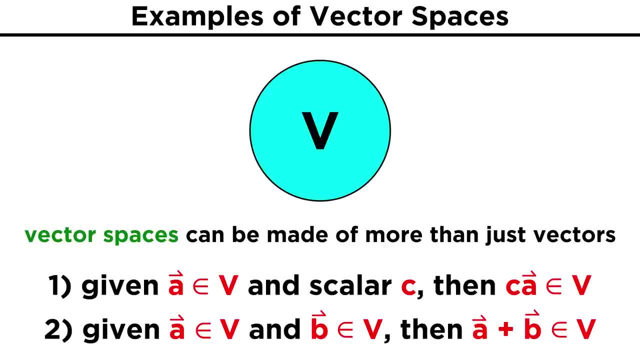 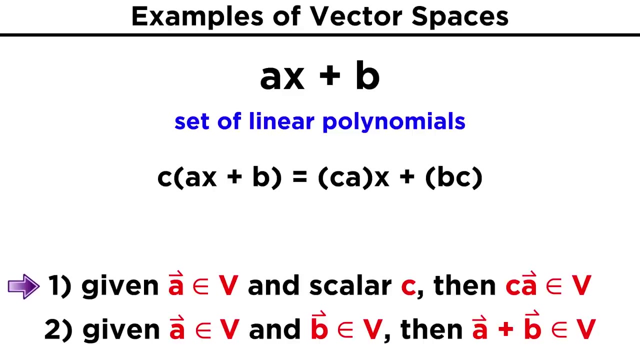 So it would seem that vector spaces can actually be made of more than just vectors. In fact, we could define a vector space that was made up of functions if we wanted to. For example, let's take the set of linear polynomials in the form of AX plus B. If we multiply by a scalar C, we can distribute to get CA times X plus BC. Since we are dealing with real numbers, CA and BC will also be real numbers. 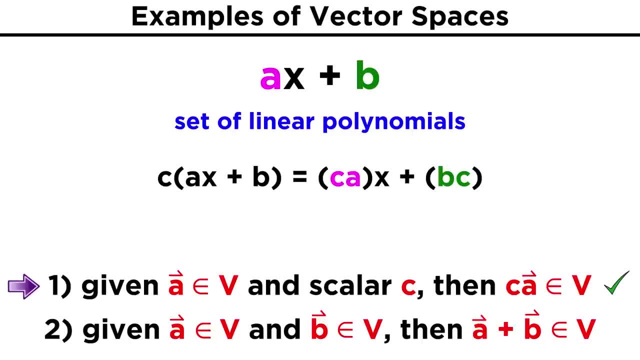 And the form of our equation is still a linear polynomial, so our result is still within the set. 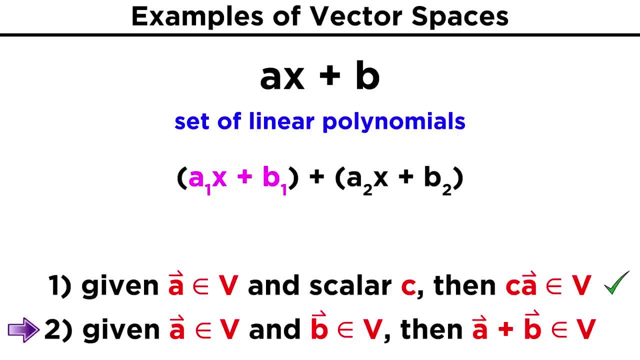 Similarly, if we have two different equations, A1 times X plus B1, and A2 times X plus B2, and we add them, once we group like terms, we get the quantity A1 plus A2 times X, plus the quantity B1 plus B2. Once again, all of these are real numbers, and we get another linear polynomial that is contained in the set. 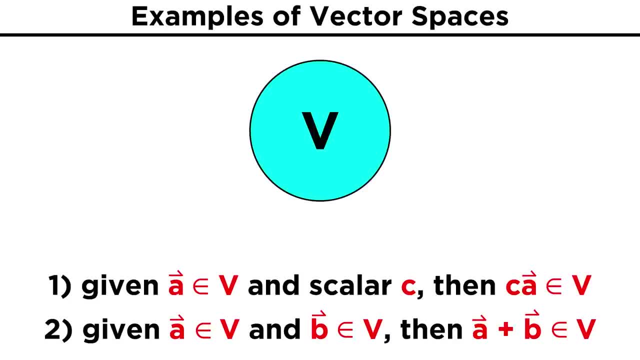 We've listed a lot of examples of vector spaces now, so what does it look like when the closure properties are not satisfied? Take for example a simple set made of vectors of length two. 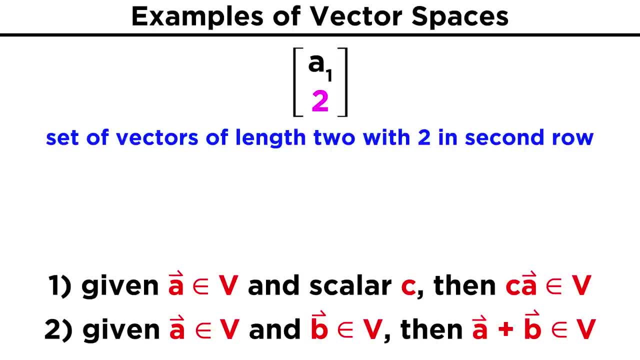 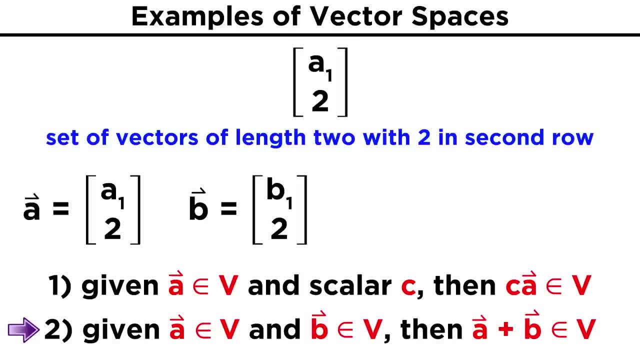 Let's take two elements of this set, A and B, and try adding them together. We don't even need to assign values for the entries in the first row to see what will happen. The first row will be the sum of A1 and B1, while the second row will be two plus two, which is four. 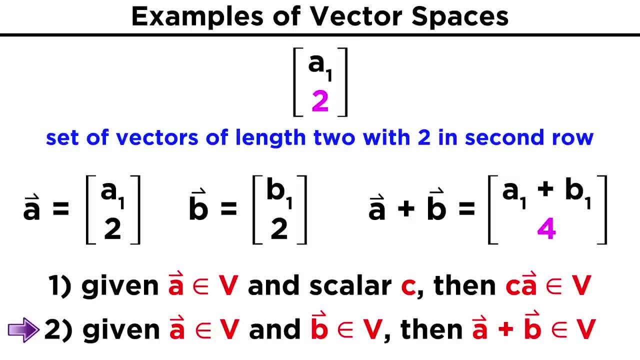 Our starting set only contained elements with the value two in the second row, but when we added two vectors of this set, we got a four in the second row, which means the sum is not a member of the set. Thus, the set is not closed, and is not a vector space, despite the fact that it is made of vectors. spaces, so let's check comprehension. 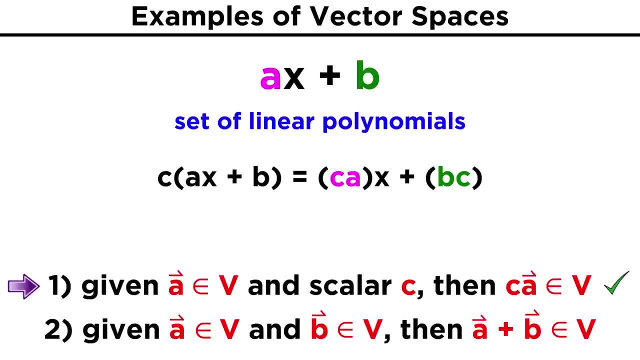 And the form of our equation is still a linear polynomial, so our result is still within the set. Similarly, if we have two different equations- A1 times X plus B1, and A2 times X plus B2, and we add them, once we group like terms, we get the quantity A1 plus A2 times X plus. 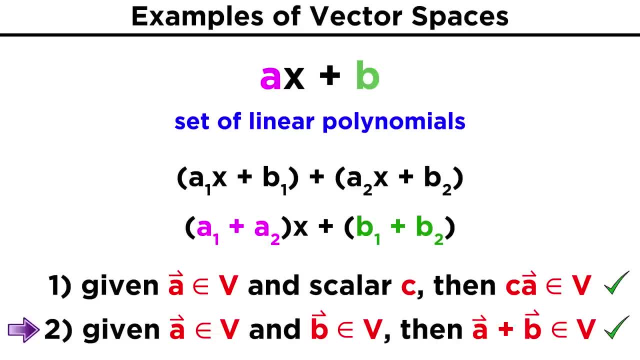 the quantity B1 plus B2.. Once again, all of these are real numbers, and we get another linear polynomial that is contained in the set. With these two closure properties satisfied, we therefore have a vector space made of functions. We've listed a lot of examples of vector spaces now, so what does it look like when? 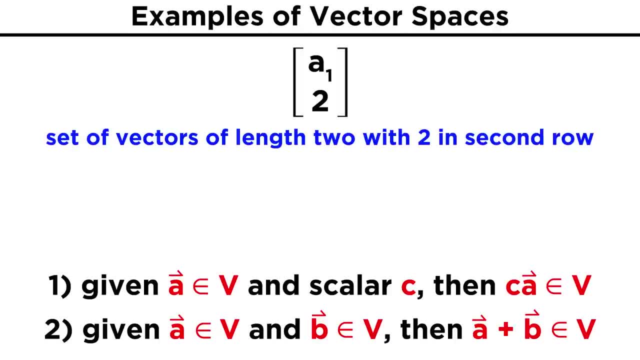 the closure properties are not satisfied. Take, for example, a simple set made of vectors of length two. however, all the elements of this set have a value of two. in the second row, Let's take two elements of this set. Let's take two elements of this set. 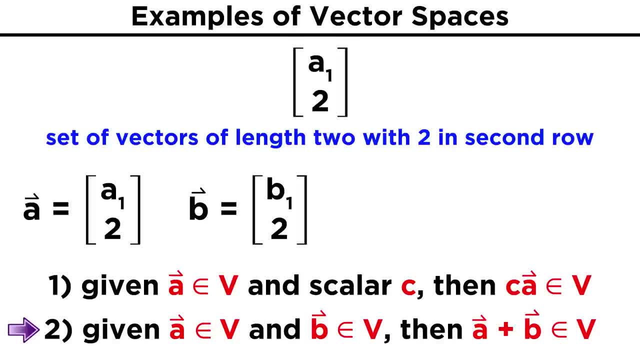 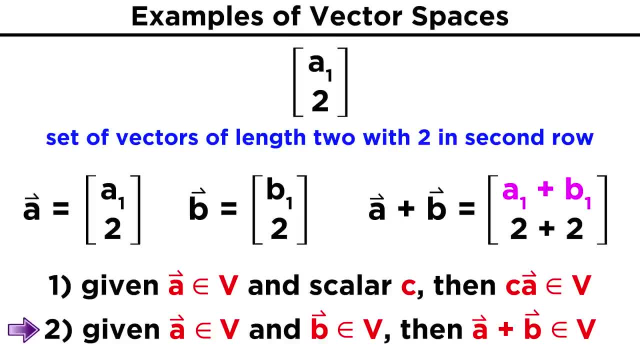 happen, The first row will be the sum of A1 and B1,, while the second row will be two plus two, which is four. Our starting set only contained elements with the value two in the second row, but when we added two vectors of this set, we got a four in the second row, which means the sum. 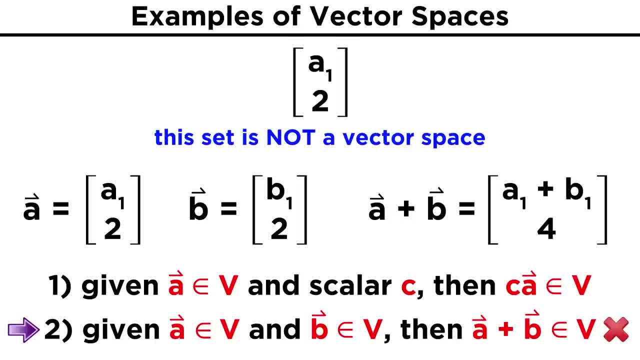 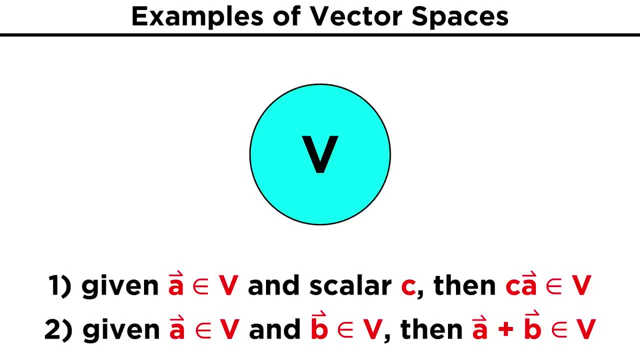 is not a member of the set. Thus, the set is not closed and is not a vector space, despite the fact that it is made of vectors. A lot of the topics we introduce in the coming tutorials will involve working with vector spaces, so let's check comprehension. 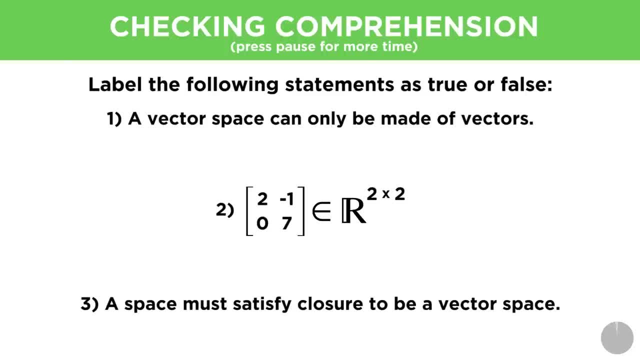 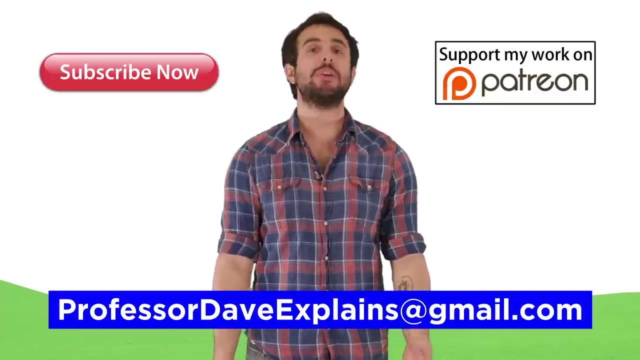 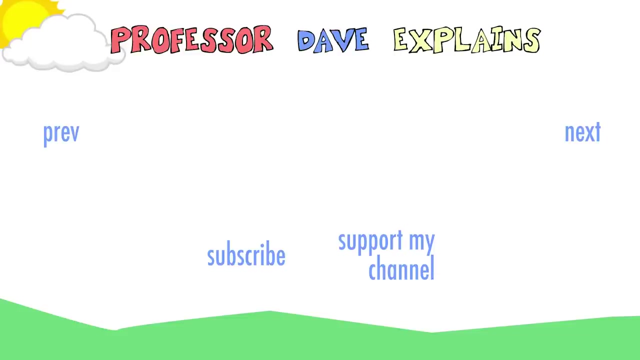 Thanks for watching guys. Subscribe to my channel for more tutorials, support me on patreon so I can keep making content and, as always, feel free to email me professordaveexplains at gmail dot com. I'll see you in the next one.